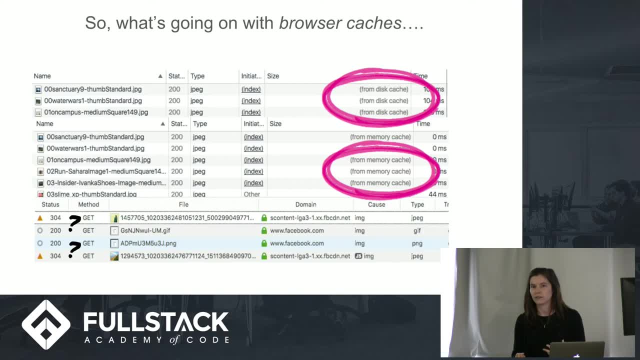 between these 304 statuses that we're getting, which means content not modified, versus 200 responses that were sent from the cache. And just so you guys know, every browser is a little bit different, So these things will change based on, sort of like, the functionality of the reload button. 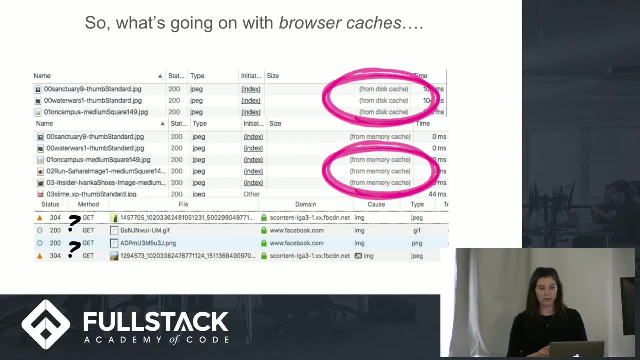 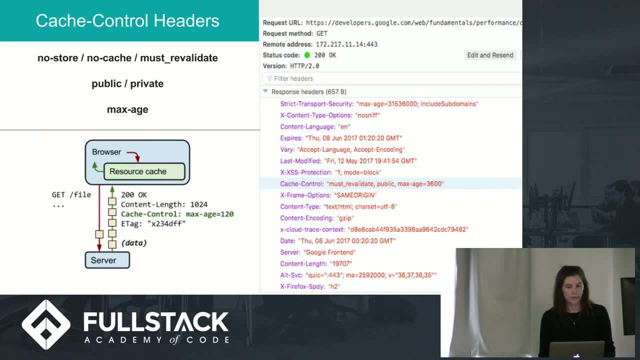 or ways that certain things are stored in memory. So, disregarding those types of variables, what can we do about that? What can we do about caching? So there are certain things that we can take advantage of, And those things are within the response headers. 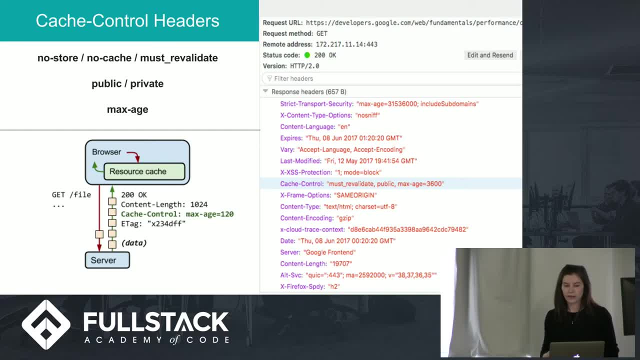 So there's this property called cache control, And there you can assign it certain attributes such as no store, which means every single time a user requests an asset, you're always going to ask the server for that particular asset. You're not going to store it in your cache. 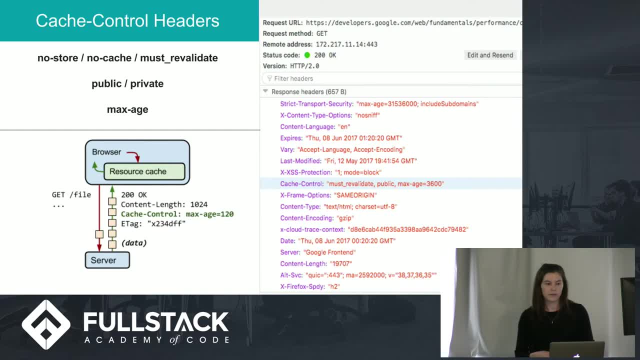 So this is for stuff that's like constantly updating. No cache is a little bit different. So again you're going to ask the server for that resource, But if there haven't been any changes since the last time you cached it, 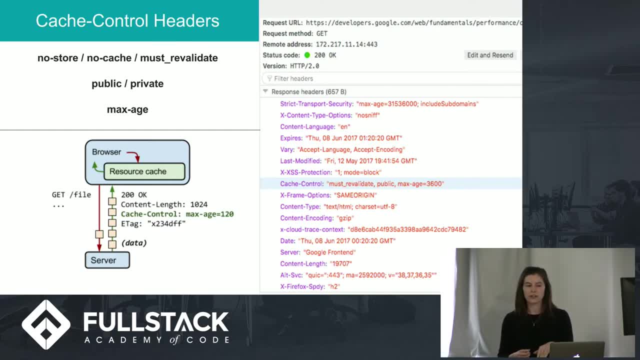 then the server will tell you to just use whatever is in the cache. So those are your 304 messages, And then must revalidate is a tiny bit different. It's only going to go to the server once it finds something in the cache has expired. 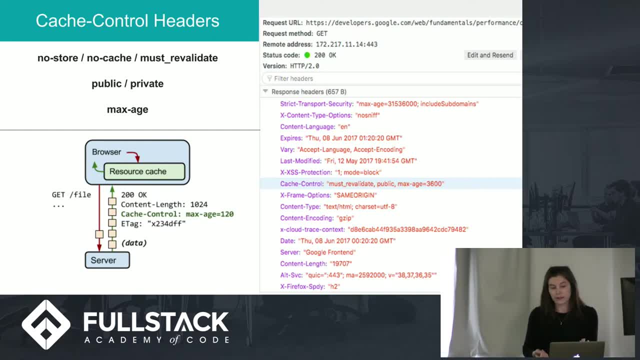 So that's sort of the standard way that a cache works. It's just a more explicit way of stating it. Public versus private. Private is really only necessary if you're dealing with very sensitive information, like a banking information, And you only want it stored on the end client's computer. 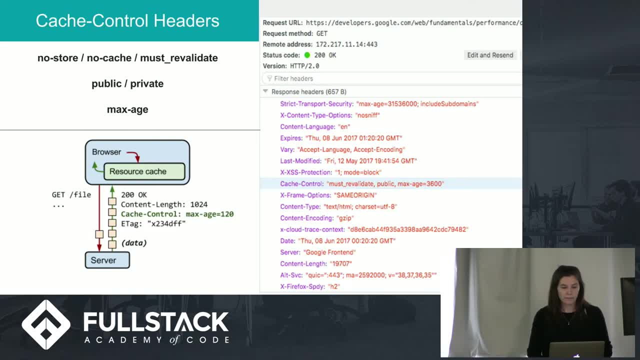 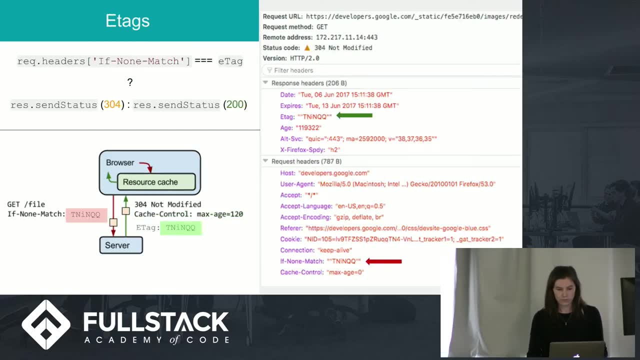 not any intermediary computers. And then max age has to do with the expiration date, So how long in seconds does it take before that resource expires? And ETags are sort of the mechanism behind comparing whether what you have in your cache is the freshest resource available. 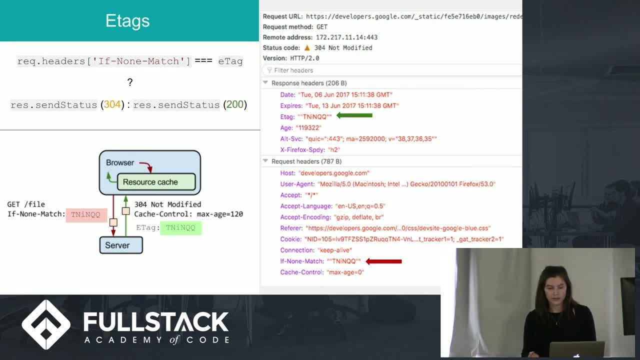 So in your request you'll send along this identifier- It's just a string- and then that will be compared to the string that's generated on the back end, And there are certain libraries for doing this And sometimes you can create an ETag from hashing the contents in the file. 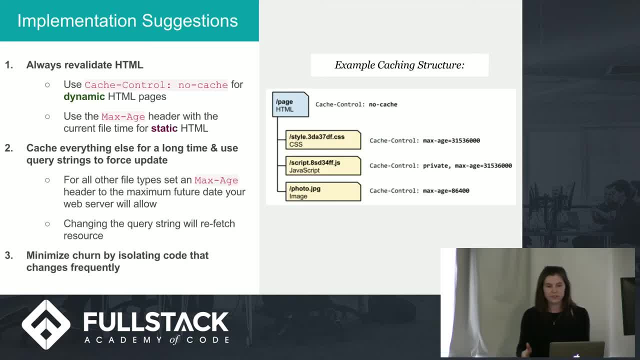 So these are just some suggestions about how to use the cache effectively For HTML. it's a good idea that you're always checking with the server to see if there's something more recent available, because you never want your client to be looking at something that's stale. 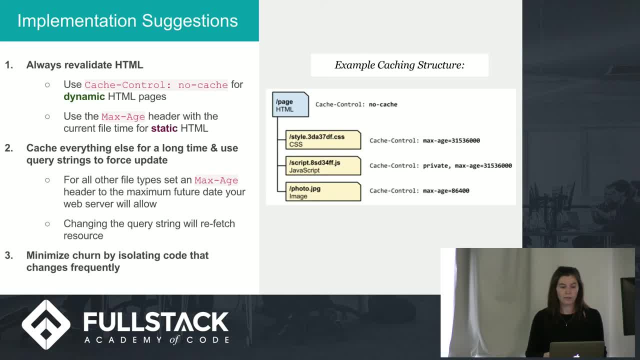 So you should be using the no cache header or determining what the max age of your document is. So that could be a few minutes, It could be hours, It could be days. For everything else, usually CSS and JavaScript doesn't change a whole lot. 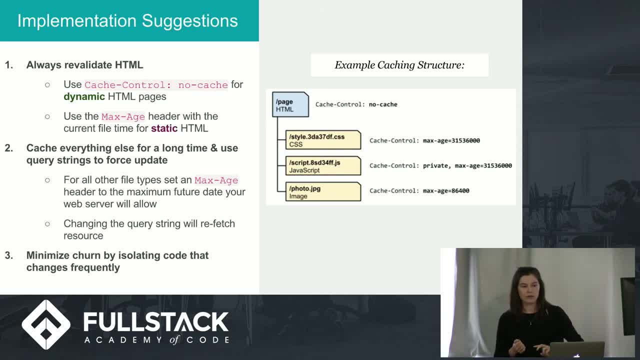 One common thing that you'll see is you'll have sort of like a string, which is a fingerprint, that identifies each of these JavaScript or CSS files, so that the browser knows it's looking for that one particular version And if you ever make changes to your CSS or your JavaScript. 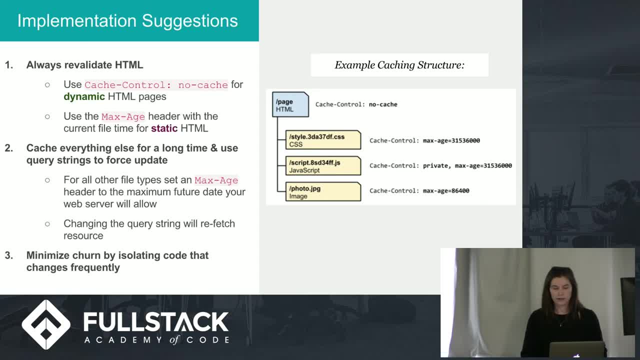 then you're going to change the string, that fingerprint, And, lastly, try to minimize the amount of churn in your application. So if you have something that changes frequently, maybe extract that out and create a new file And that can be cached frequently versus something else. 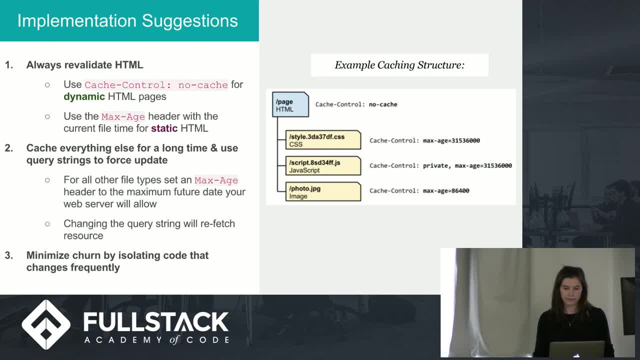 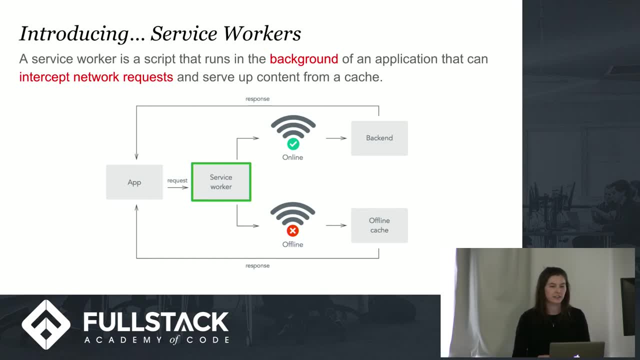 that needs to be saved for a long time. So service workers is a new sort of technology. It's a JavaScript web worker and it runs in the background. It runs in the background of an application and you probably have a lot of service workers. 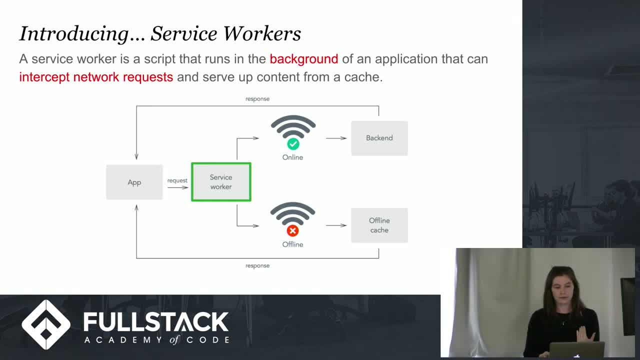 that you're not even aware of right now. So service workers act as sort of like a proxy server. So when you have any inbound requests from your client, your service worker will intercept those and it'll see if it has any of those assets in the cache. 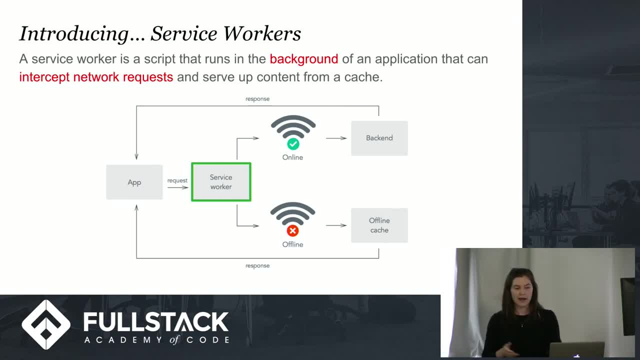 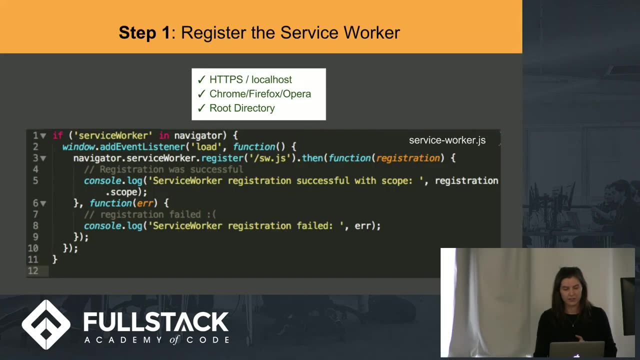 If it does, it'll send them back. If not, it'll pass along that request to your back end. So it's really good for if you're designing around an offline experience or when a client doesn't have a good connection, And I'll demo this in just a minute. 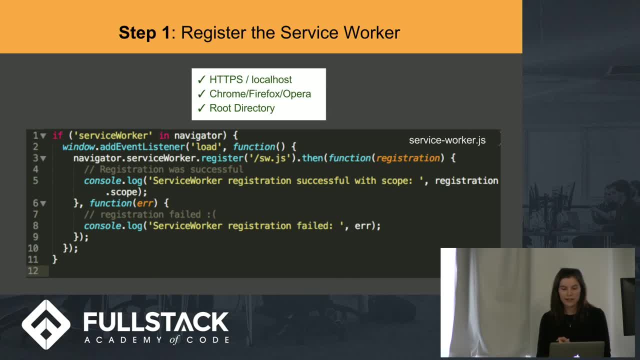 There are some prerequisites that you need. You have to have a secure connection or be on local host. You have to be using one of those browsers there And also, when you register a service worker, it needs to be in your root directory so it has access to all the underlying files in your application.